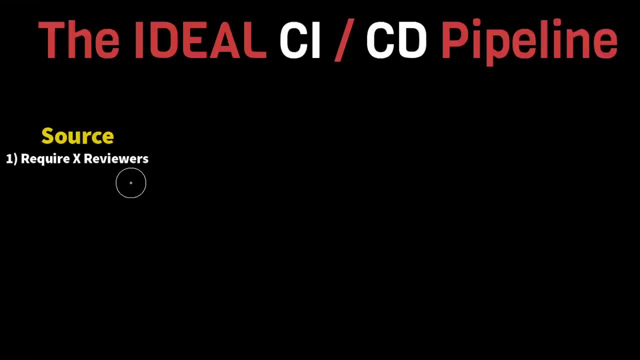 be configured using a lot of different technologies, but I think this is a definitely a required step. At a minimum you should have one reviewer, but probably a safer bet would be to have at least two, But personally I wouldn't go over that. So the source step isn't really. 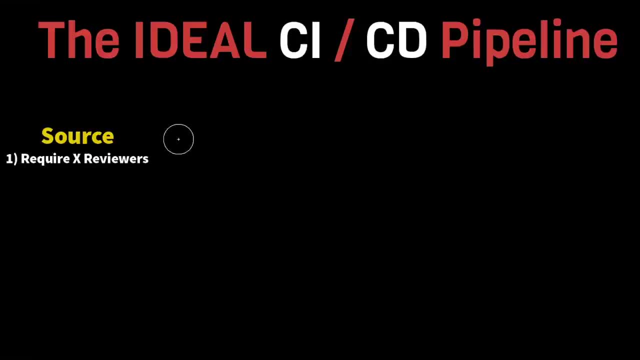 interesting and there's not really a whole lot you can do here, So let's move on to the next step now. So the next step is in terms of the build process, And this is after you commit a change to your source code. it's going to automatically go into the build step And what's included in 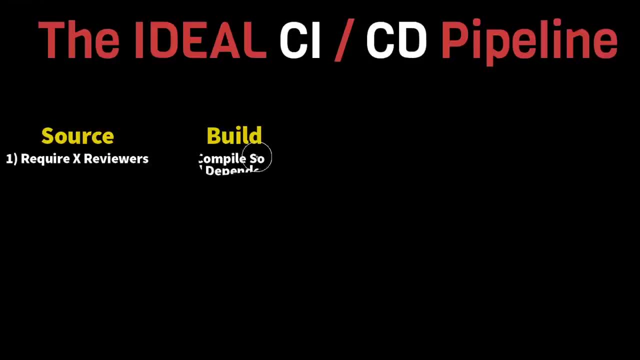 the build step. What are the actions that you should have associated with it? So the first one is a pretty obvious one again, which is just to compile your source code and all of your different dependencies. So, whatever's in your build process, you're going to have to compile your source code. 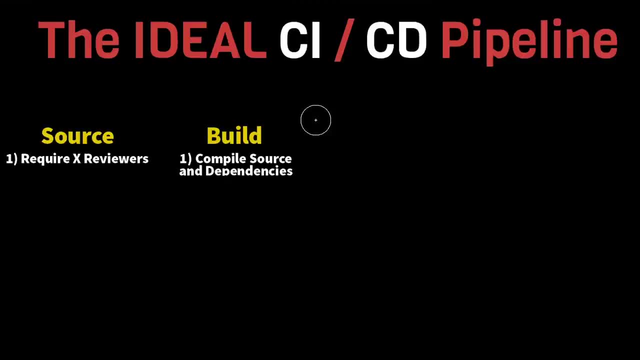 packagejson or your palm file or whatever language you're choosing. You need to be able to compile all that source code and all the dependencies that are included in your project. The next step is that we need to run all the unit tests that are associated with your project. 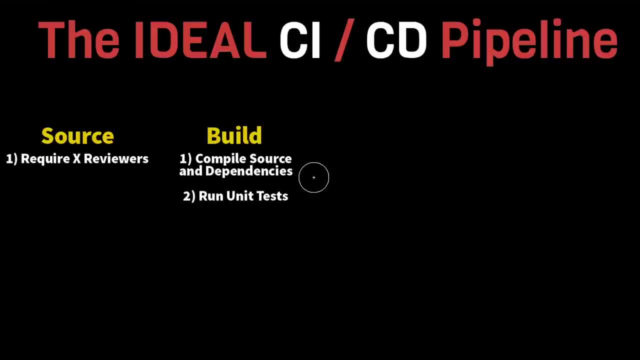 So ideally, if you're going to have a CI CD pipeline, you need unit tests and you need a high coverage level of your unit tests. So a lot of different tools these days show you like whether or not a line of your code is being tested by unit tests, So take advantage of that. However, 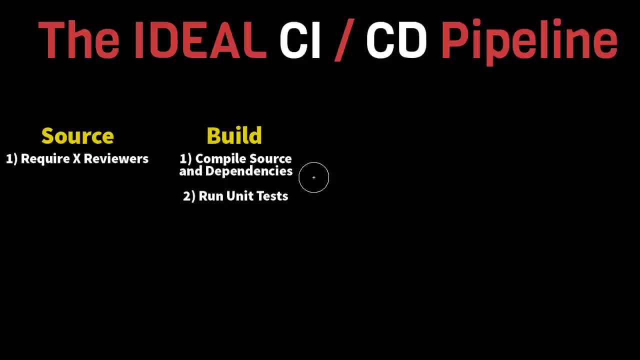 if you want to have a CI CD pipeline, the whole goal is for you to be able to basically blindly push a commit into your source control and be confident enough that it's going to be caught at one of these later steps in the process. And if you don't have unit tests and you don't have 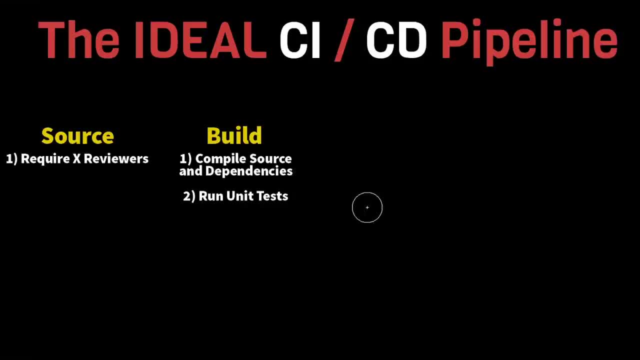 high coverage on your source code, then it's just going to flow all the way through to your next stage And then you're going to have errors You're going to need to roll back. It's going to be a pretty painful process. So make sure that you have unit tests and you have a high level of unit tests. 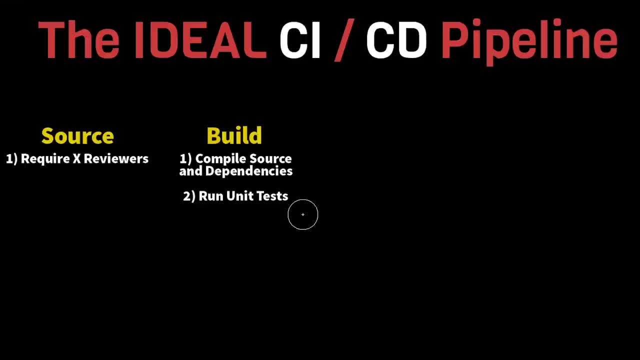 to be confident in how your application is running and that it's working correctly. Now the next step is code coverage And this kind of ties into what I just spoke to. So a lot of testing frameworks such as TestNG or even JUnit, output the code coverage percent. 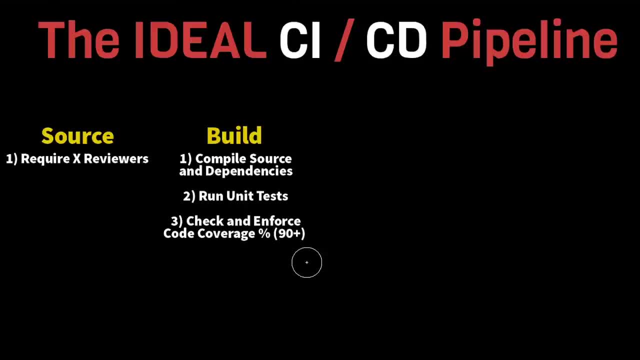 And that code coverage percent of that specific commit is going to be important. So ideally you're going to want to have a minimum of 90% or so, And any subsequent commit should not be lower than this threshold as well. So this should always be an increasing. 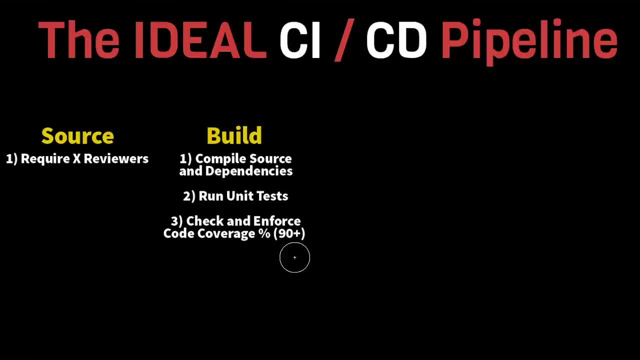 number. I know a lot of people don't strive for 100% because it becomes meaningless at a certain level. But you can always try And generally a higher number is usually better, All right. So after that we have our first kind of environment And that's going to be our testing environment. 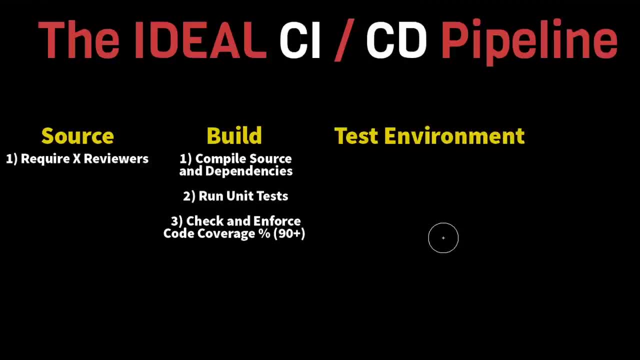 Now your testing environment is going to be where you're testing your changes to be comfortable that they're ready for the next stage, which is something closer to production. Now the primary thing that I do in test environments as a prerequisite to the next step is to run my 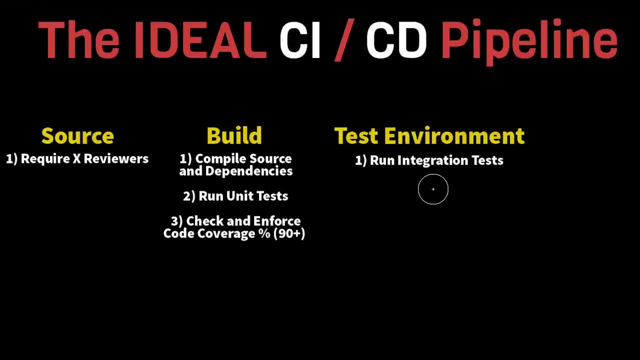 integration tests. Now there's a lot of folks that have different interpretations of what integration tests mean and how that compares to functional tests, And there's a whole debate over what the correct terminology is. But let me just tell you what I'm talking about when I say integration. 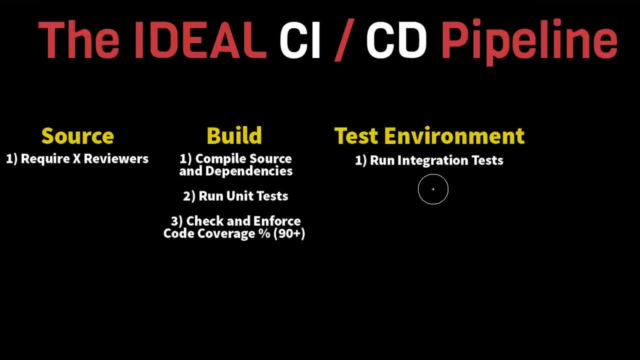 tests. When I say an integration test, I mean if you have an API such as create order, you should have a test that executes the create order API and ensures that the correct outcome ensues. So, for example, in this hypothetical integration test where I'm testing this, 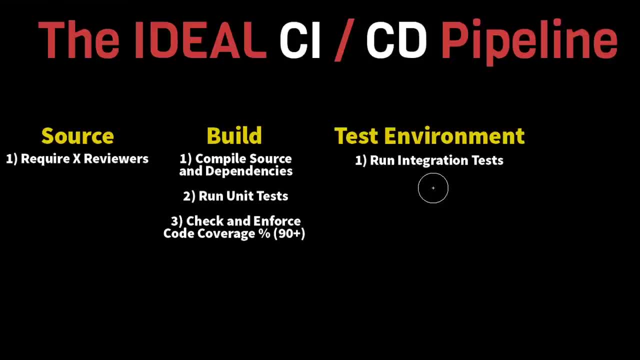 create order API. after I call that create order with an expected input, I should also call get order right after that And I should look at what the order contains. Does it contain all the things that I set when I created that order? If it doesn't, then there's something. 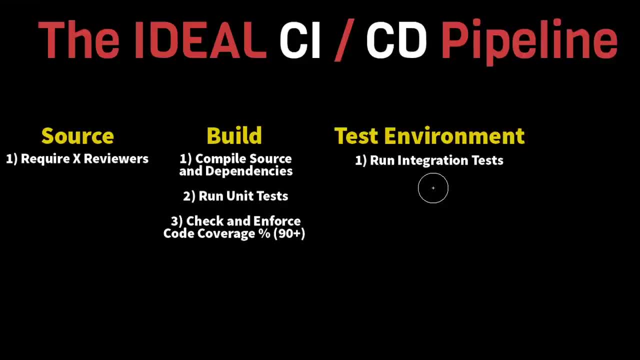 wrong. If it does, then you pass that test, Congratulations. Integration tests also test the behavior of your application in terms of business logic. So, for example, if you have a create order API and there's some business rule in your application that says you're not allowed. 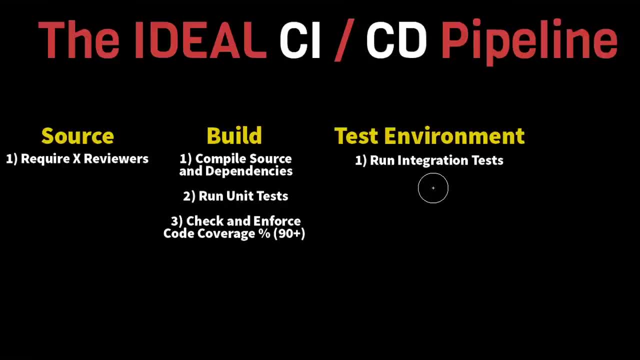 to create an order where the dollar value is over, let's say, $10,000,, you should have an integration test that tests that functionality, because that's an expected business rule. So it's not uncommon to have like 50 to 100 integration tests, depending on the size of your. 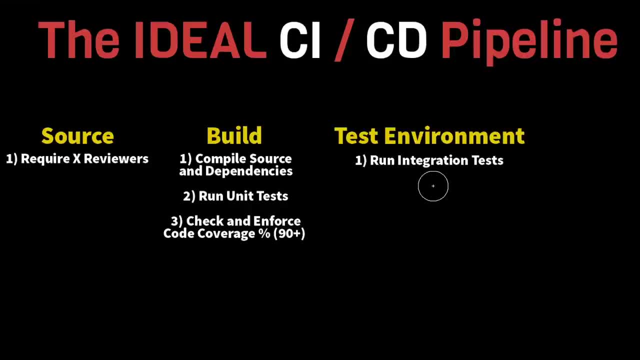 project, But really this is where you test the core functionality of your APIs to see if they're doing what you're expecting. Now, one thing that I do want to add, and let me just get my pen here to talk about this section a little bit more. but you should have the ability to turn these on and 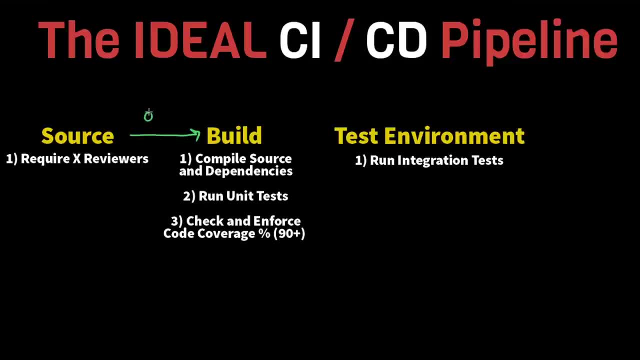 off. So the fact that you go from source to build should be kind of a switch that you can enable or disable at any point in time, Because you know there could be a case where someone pushes something. you don't necessarily want to build it right away. Maybe you want to do something over. 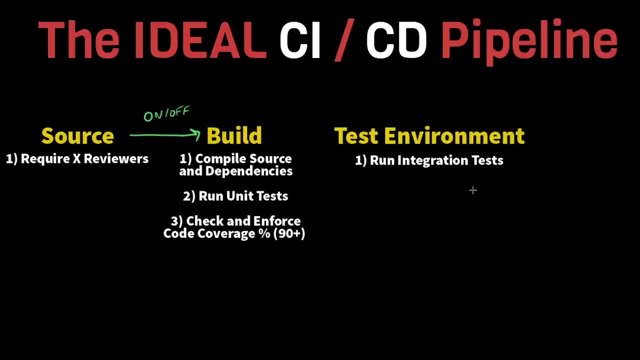 here, or there's something that's in the pipeline and someone's testing something and you want to make sure they can finish before you start deploying your change. So ideally you should have the ability at every stage to turn these like on and off, so that you can control what gets. 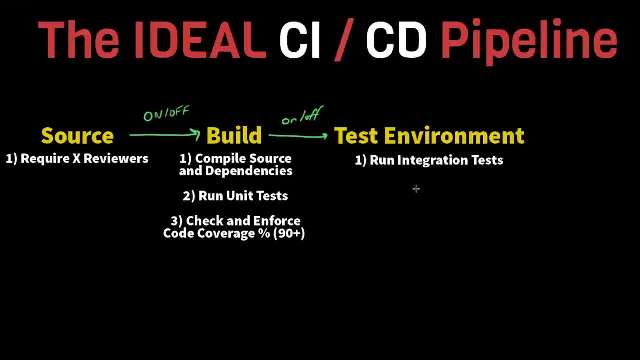 promoted to the next step of your deployment pipeline. And one thing that I also wanted to add is that in the test environment, like when you're running your integration tests, if you also have other dependencies- like, say, we have order service, which is responsible- 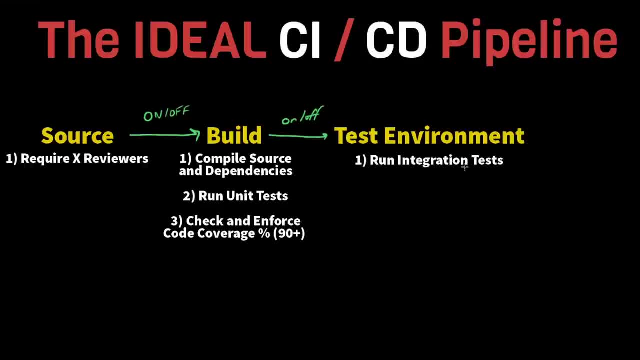 for creating orders. you may have other services that you depend on, maybe a service that manages all the addresses for your customers, or maybe a service that stores all your customer profile information. If there's dependencies in any of your APIs, you should also be testing those things. 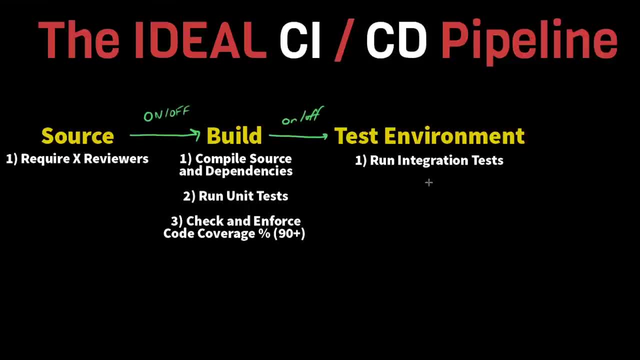 as well. So if create order has a dependency on a customer profile service, when you run your integration test for create order and it depends on that customer profile service, you should also be testing that you're getting the expected information back from the customer profile. 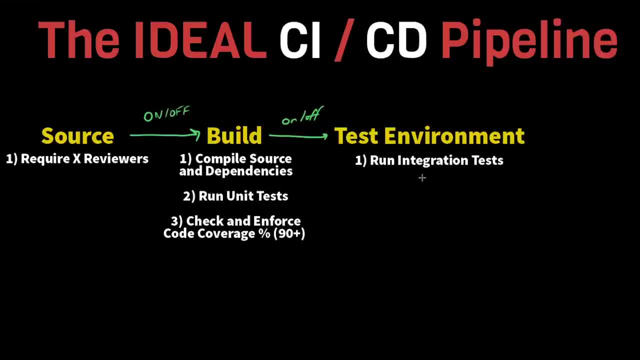 service. So this kind of tests the end to end workflow of the system And it gives you a lot of confidence that all your core APIs and your core logic is working as expected. So that's the core idea for the test environment And this is really where you're going to spend most of your 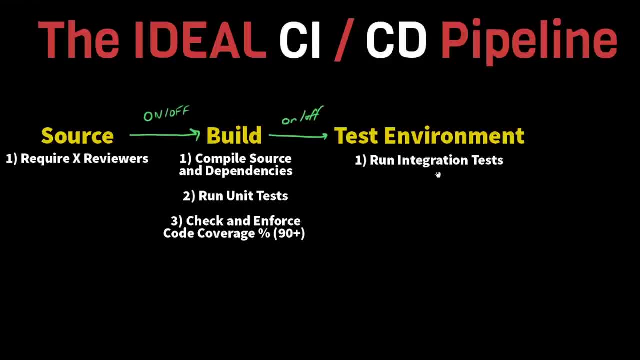 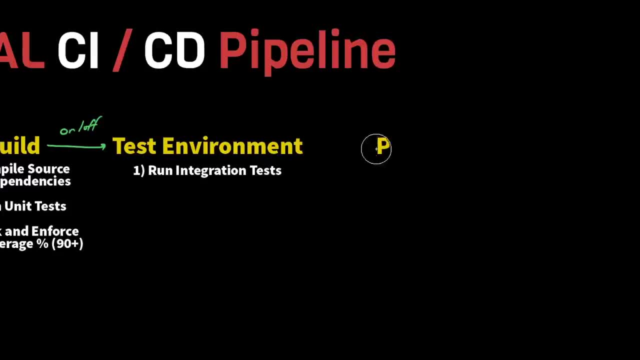 time It's your sandbox to basically try things out. Now the next stage is: usually I have a another stage in between test and production, But in this case, I decided to just keep this as a production environment. Now, one optional thing that I wanted to point out is: 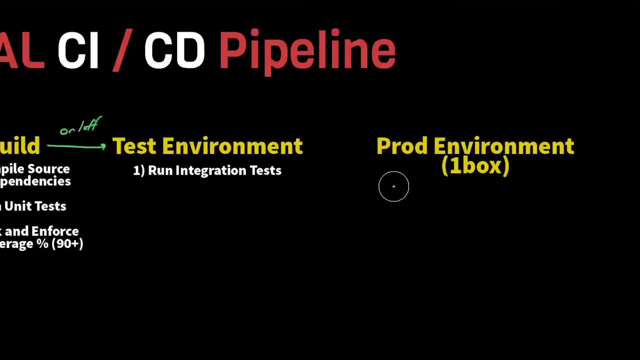 that if you have a kind of a small to medium size organization, then having a test in a prod environment is probably going to be just fine. However, the larger your organization gets, the more environments that you may need. So you may need a test environment and then a pre. 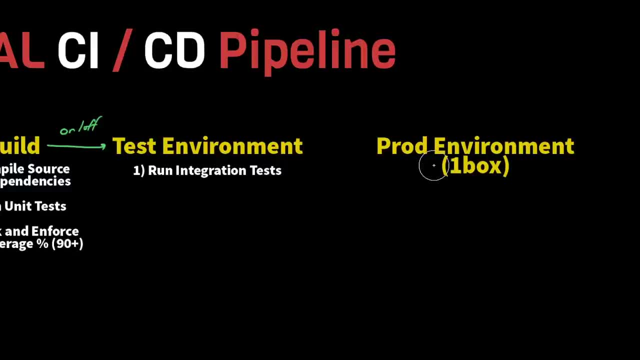 production environment and then a production environment, And this is just useful, because sometimes there could be many different folks that are testing different things at different times, such as QA, or you know someone's testing a specific feature and you need to put a branch somewhere for. 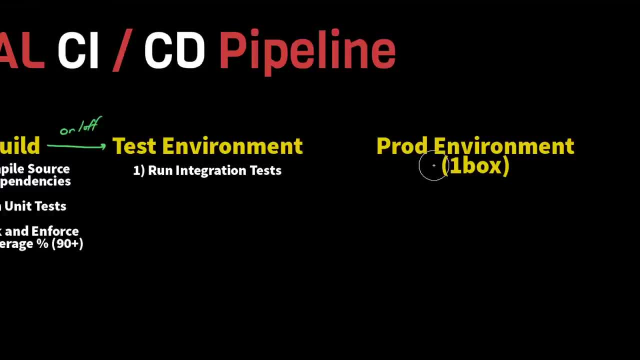 specific testing, then that's where having these additional environments will help. But if you're a small organization, two is probably fine for you, So I wouldn't really worry about it too much. Alright, so prod environment. So now we are in production And the idea of one box. 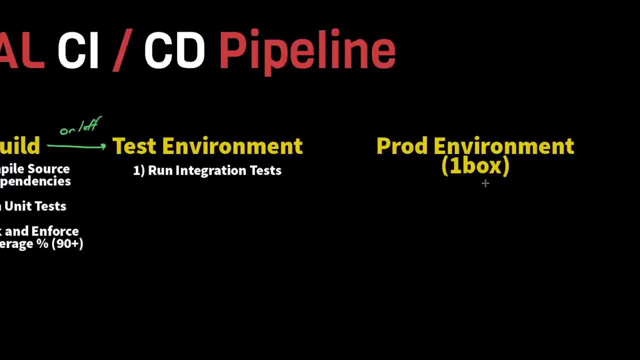 a lot of people ask, like, what does one box mean here? So a key thing that you can do to ensure that you're not deploying kind of a bad change out into your full blown production environment where all your hosts are located, where all the traffic is going to be hitting for your customers. 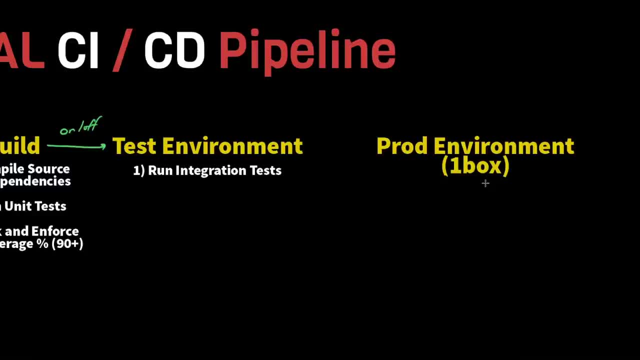 is that you have this idea of one box And basically what one box represents is that it's a fraction of your production traffic. Okay, so say you have 10 hosts in your production environment, you may have one host. that is the so called one box host. So really this should be. 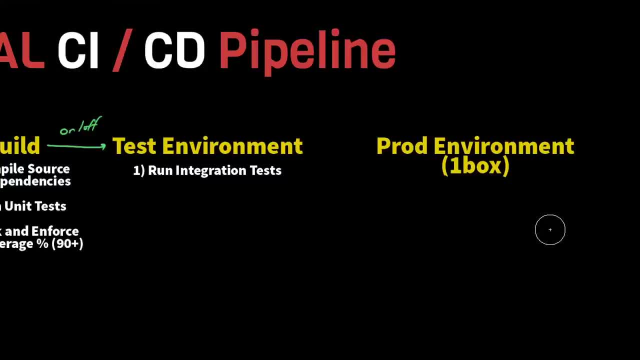 something like 10% or even less of your production traffic. So you're going to have 10 hosts in your traffic And this just gives you the confidence, such that you know if you detect that there's something wrong on this host, like maybe your alarms are going off, maybe your latency is really. 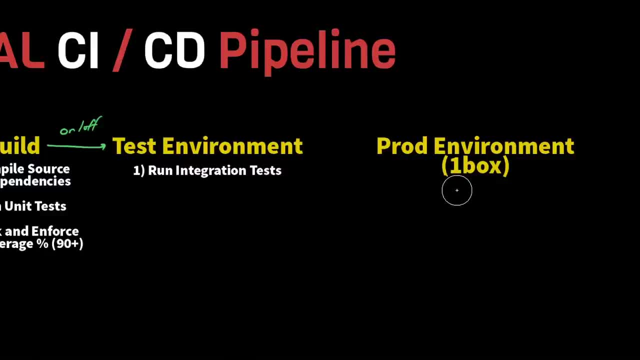 high. when you promote this change from your test environment to your prod one box environment, That means that you know this is a bad deployment and you need to roll back that change right away. If you went from test to your full blown production environment all the way over here on the right, 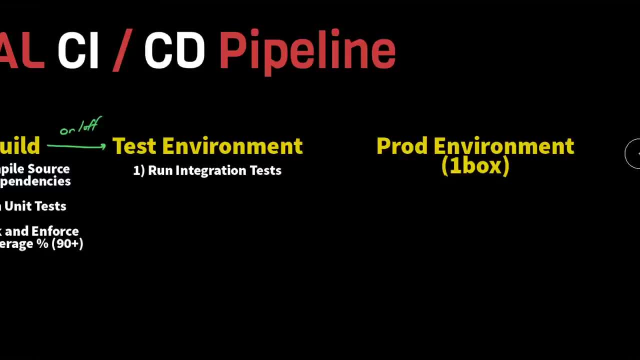 then that means that you need to roll back like 10 or 20 hosts in your environment, And that's going to take a really, really long time. So you're going to have to do a lot of testing, Whereas if you just needed to roll back one host in your one box when you detected there's a bad 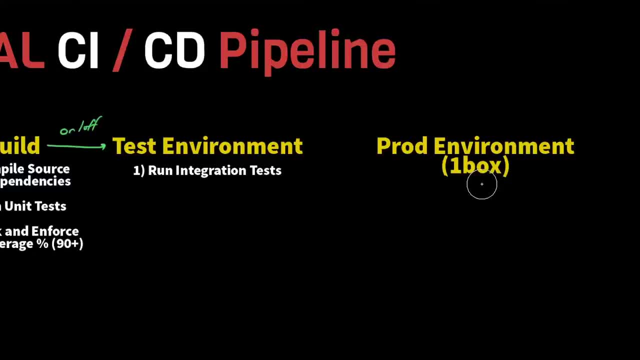 deployment. that's a pretty straightforward process. It's really fast. you just disable that host And the previous version of your code is going to be in your production environment and there's going to be no harm done. So that's the idea of one box and why it's such a powerful. 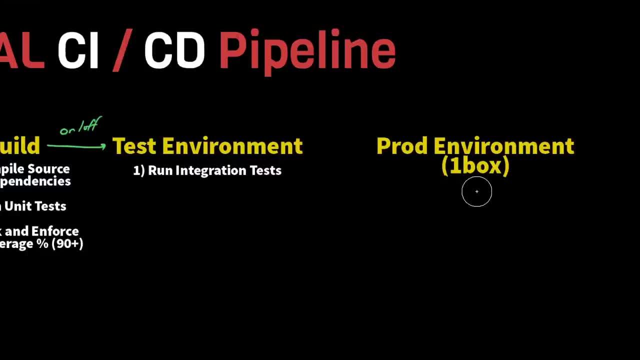 tool. I'm not sure what other people call this in the industry. This is just kind of what I call it and what a lot of people in my workplace call it, But this is definitely saved my butt a lot of time And a lot of my coworkers times, and I just think that this is a critical step. 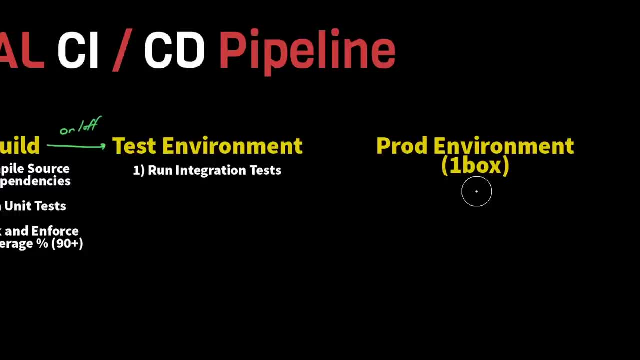 in any CICD pipeline to be comfortable with your change before it hits production. Now, if you're in a full blown CICD pipeline, you probably don't even care about this anyways, because you're going to be so confident in your integration and your unit tests that you're going 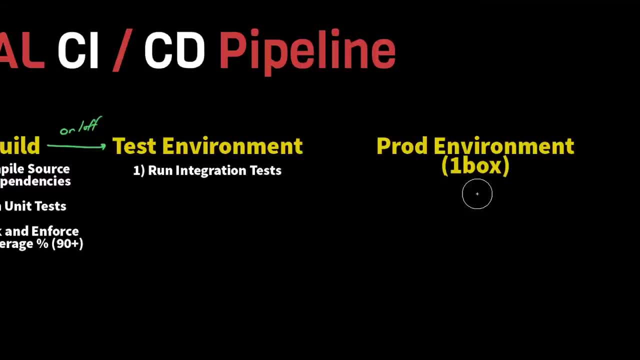 to be safe, to go basically directly to prod. But most of us want that extra layer of kind of safety net I want to say. So that's where this one box step really comes into play. All right, so when you deploy your change from your production environment, you're going to be able to see 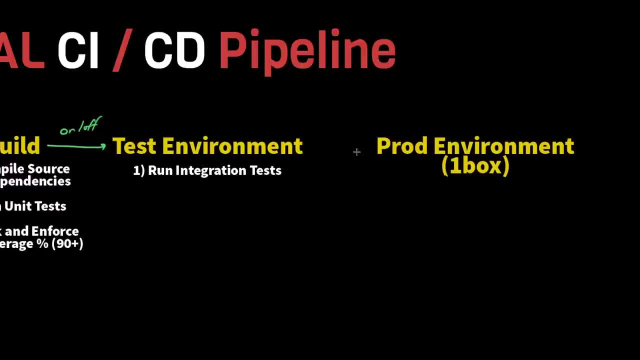 from test environment and let me just draw this out really quick again. So test environment over here into production. there's going to be many things that can go wrong in this deployment right. There could be an elevated number of errors, there can be latency spikes, there could 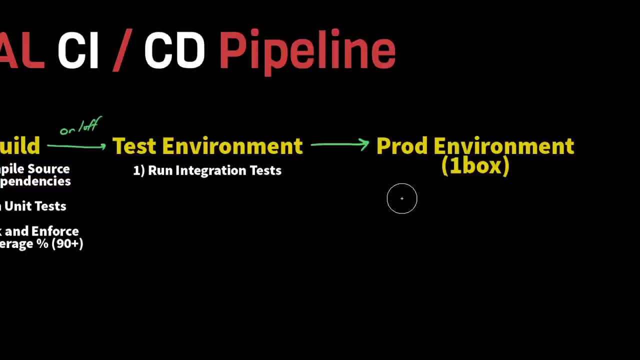 be key business metrics that are faltering. maybe the numbers of number of orders that are being created start to drop very rapidly, And that's a very abnormal pattern. So what you really really need in your prod environment and one for specifically one box. 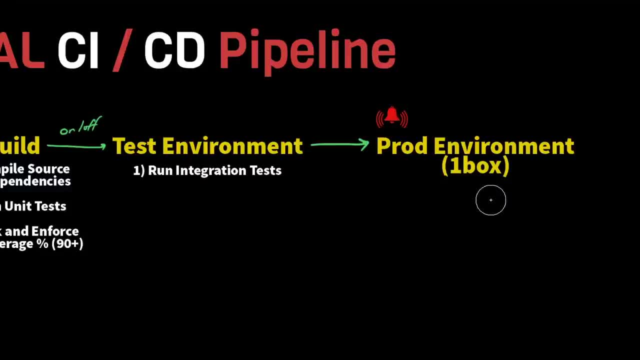 is this concept of alarms and, more specifically, rollback alarms. Now, rollback alarms are basically an alarm type that monitors a particular environment And during the deployment step. like this alarm would be integrated in this deployment process And you would monitor very specific things about this particular deployment and this version of software for things like 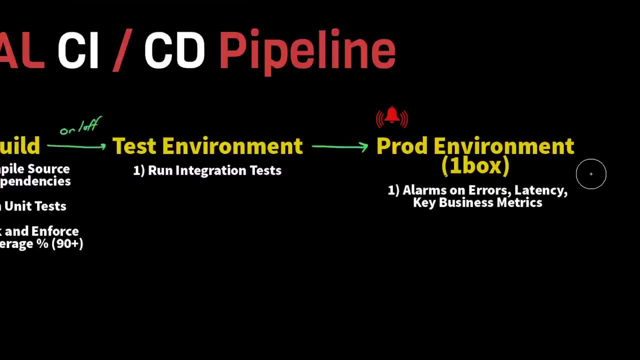 errors, latency and your key business metrics. These are the key items that should be integrated in that rollback alarm And if anything here, anything in terms of errors, gets elevated, if your latency gets elevated or your key business metrics start dropping below a known threshold that's deemed to be healthy, 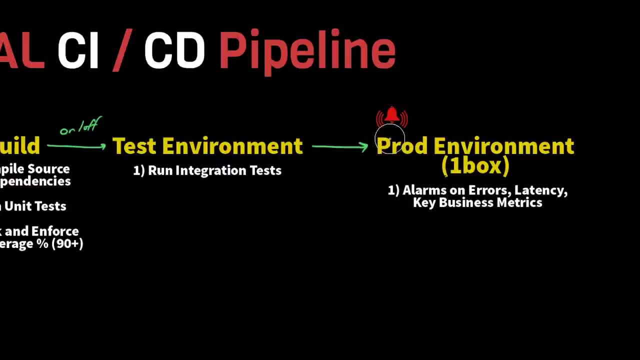 then that's an indicator that you should probably roll back this change Now. a good CI CD pipeline will directly be monitoring these types of metrics that you configure on the environment, And this rollback should happen automatically. There shouldn't be a step that you need to do. 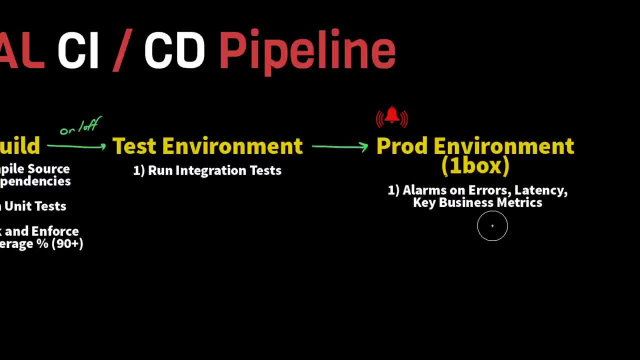 manually. there should be something that is automatically baked into the system so that it can monitor these metrics, And if you're not familiar with CI CD pipeline, you should probably monitor these metrics and roll back when it determines that any of these metrics exceed a. 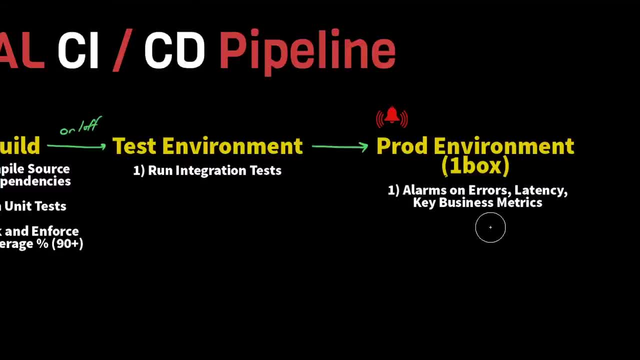 threshold, All right. so assuming that that was fine, that you got through the deployment and none of these errors, latency or key business metrics start to drop, then your next step is kind of a confidence building step And I like to call that what is called a bake period And the 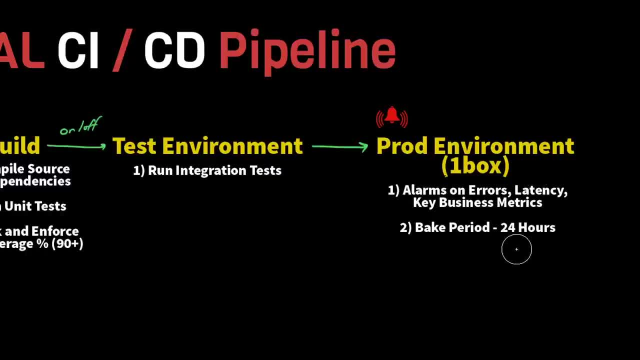 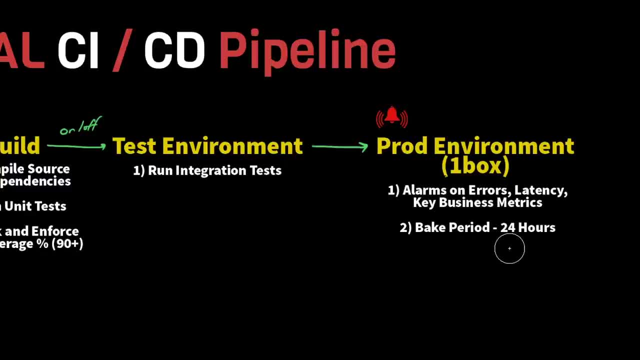 such as like mid afternoon or something like that, then you can probably really reduce this number down. However, your bake period is basically just you testing like: is this change still good? it's out in production And sometimes things may not happen right away. right your errors may not. 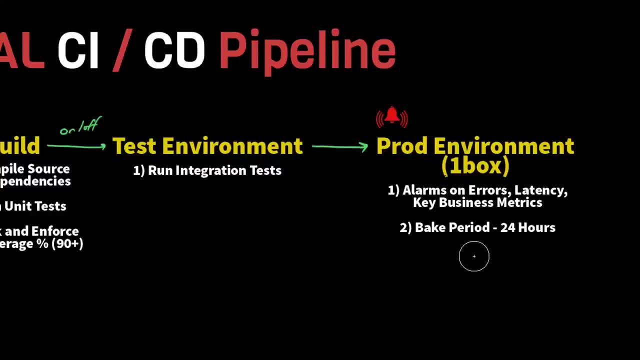 rise. your latency may not rise, something may be delayed, and maybe a certain behavior of your APIs or a certain code flow of your APIs isn't being hit until a certain system calls it, or a certain time of day, or something like that. So that's why a bake period is important here, to 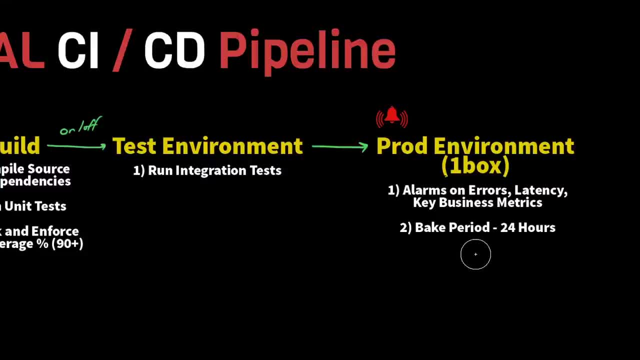 be confident that you let your change sit for a period of time And then, once it sat for that period of time and nothing abnormal has happened, then you're safe to go to the next step. So the things that you want to monitor here you can use anomaly detection, which I think can be overkill. 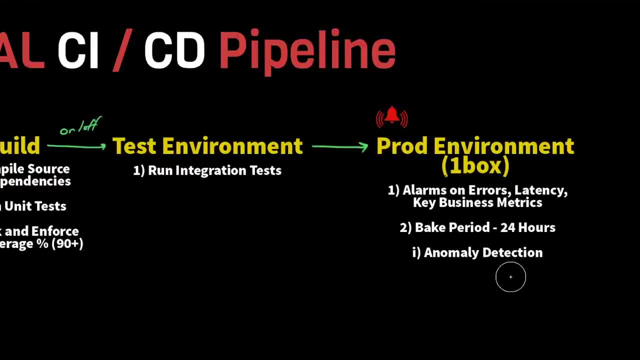 for a lot of systems And it can be a little bit expensive to- let's be real- But this is kind of what I like and what I use in my systems. However, if you don't want to use anomaly detection, there's a much easier way And it's kind of similar to what we had a number one which is: 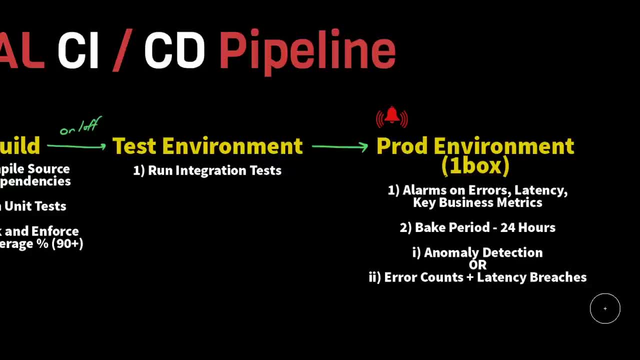 just that you monitor the error counts over a period and latency breaches over a period And, similar to what you did over here, you just kind of persist those monitors and, over a longer period of time, now start to monitor these and sum all of them up over that timeframe And if you exceed a 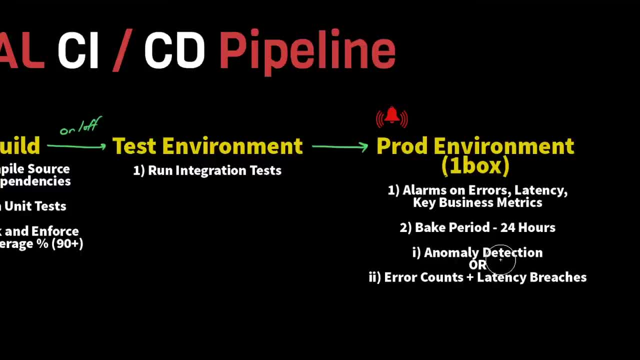 certain threshold, then you automatically roll back again. So that's how that flow works. Now the final step, which is it's not necessarily associated with this environment, but it runs on production, is this notion of a canary- And again, people call this a different name, I think in the industry, but let me tell you what I mean. 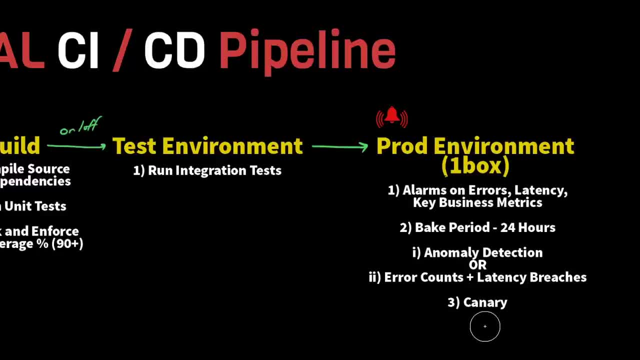 when I say canary, So a canary is just something that tests your production workflow on a consistent basis, with an expected input and expected outcome. So back to that create order API that we were talking about when we were testing it in the run integration test environment. What you would do. 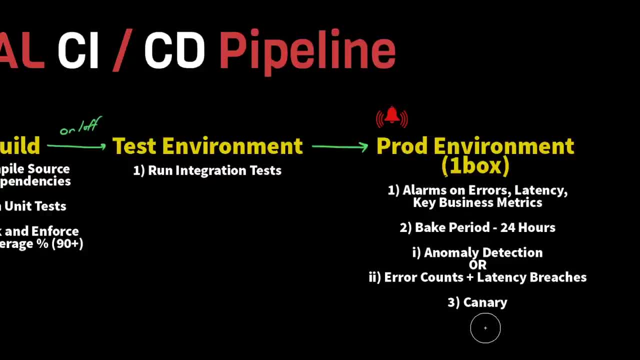 if you want to set up a canary on that API is that you'd set up, basically, a cron job that triggers every minute And inside the function of that cron job you would call the create order API with an expected input and you would hard code an expected output And you would 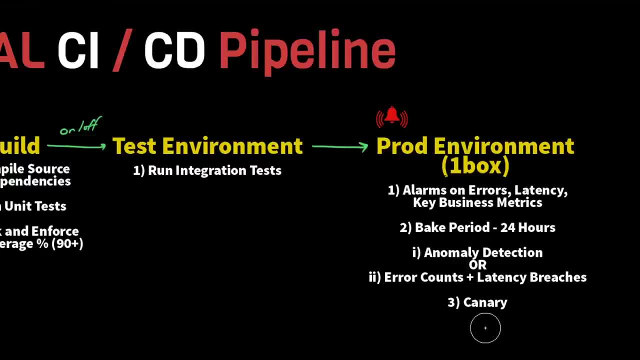 continuously call that API every one minute or possibly even less, And the idea here is that if this API ever starts failing or the output of the API starts resulting in an error, that's an immediate indicator that something is wrong with the system. So if you're using a canary, you 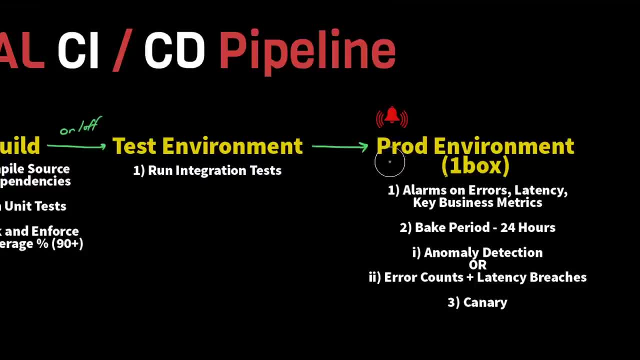 should be able to detect it right off the bat, Because if you have a new code change that gets into your production- and this canary is running constantly, 24 hours a day, every minute of the day- then anytime a bad change gets into production, this canary should be able to detect it right. 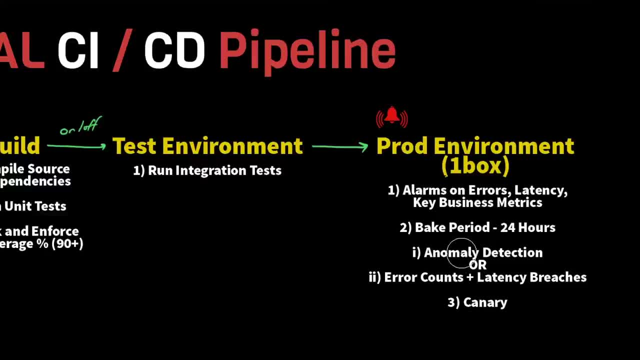 off the bat And so this kind of goes into the bake period, it goes into the key alarms and the key things to monitor And it goes ultimately back into that rollback alarm that's going to be used to kind of roll back our changes to the previous software version. So if you're using a canary, you 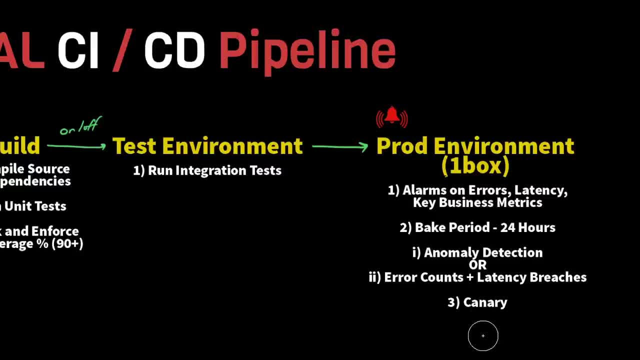 should be able to detect it right off the bat, And if you're using a canary, you should be able to. So that's the idea with the canary. It's basically a function that runs on a interval that just repeats itself over and, over and over again, And the expected outcome is that it consistently works. 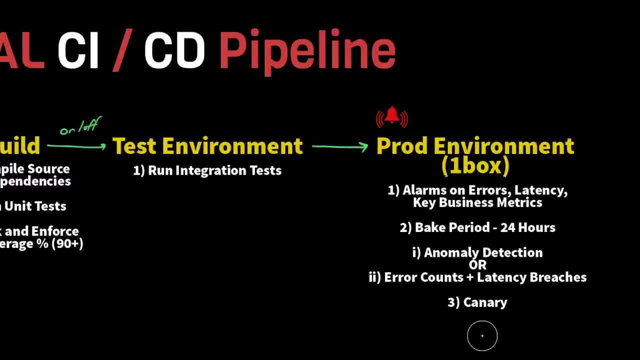 as expected. And the moment it doesn't work as expected, you trigger an alarm and that alarm triggers a rollback And that rollback moves prod back into the previous version of software that was assumed to be working correctly. So that's the key idea here. So, assuming- 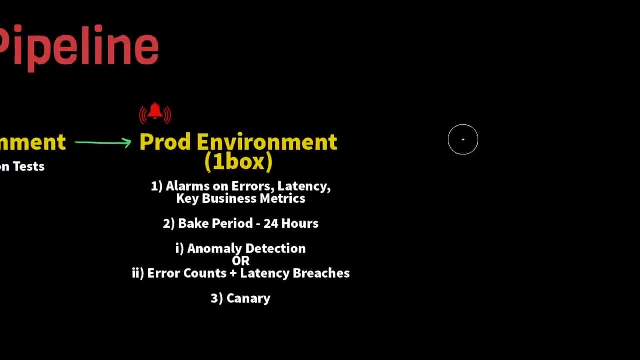 everything went well here. you're pretty much good to go to the next step, And that's going to be your full blown prod environment. So if this one box environment was hosting 10% of the traffic, then your prod environment would be hosting the 90% of that traffic. So basically everything. 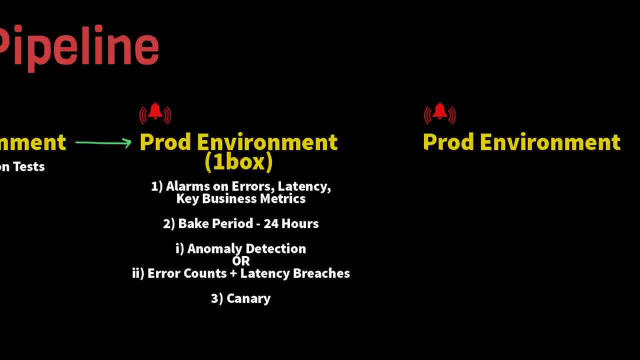 that's the remainder and everything that is over here- And actually let me just draw that out just to make it perfectly clear- Everything that is here, all of this stuff- alarms on key metrics, bake period, anomaly, detection, canaries- this should also be over here like basically verbatim, So you should have the same. 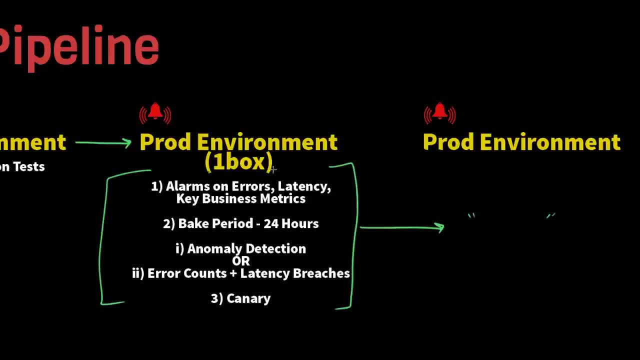 kind of checks that are running both in your prod environment and in your one box environment. One thing that I realized I forgot to add, like: how do we do this? How do we only direct 10% of the traffic to this host and 90% over here? There's many different ways. you can do this at the DNS. 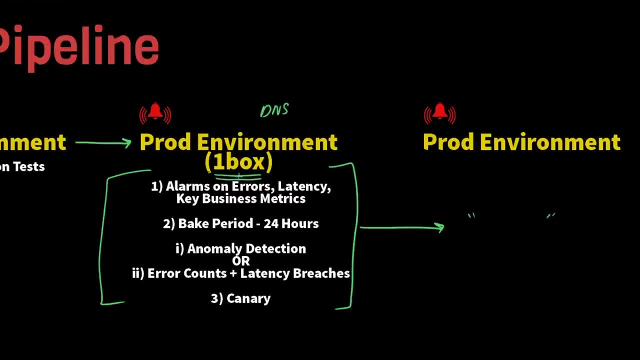 level with DNS weights, to say, 10% goes to this URL and the other 90% goes to this one. There's also other ways, depending on the technology that you're using. I know that, like in AWS Lambda, there's a weight factor that you can give to your function versions, So you can say: 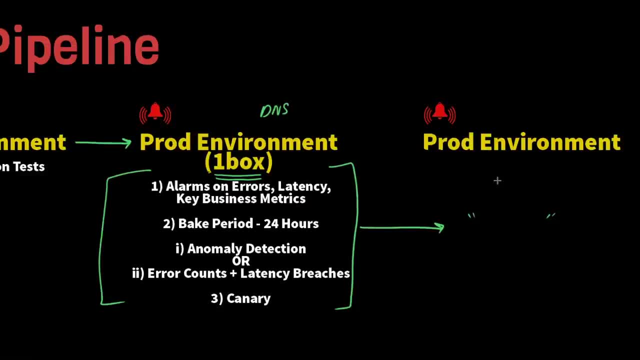 like 10% goes to this one and 90% goes to another one. That's another way to accomplish this, but there's many different ways. I'll leave it to you to look into it, but probably DNS is the most common one And that's generally what people use. So, again, everything is repeated over here and you 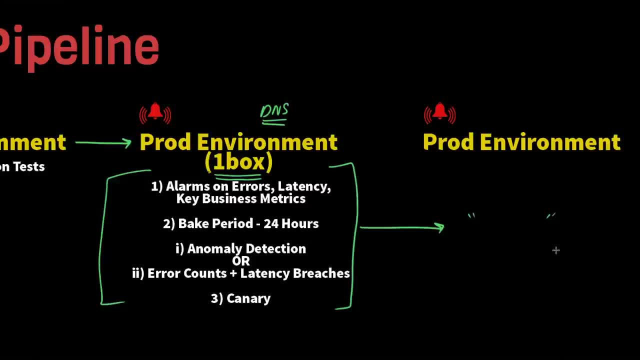 have all those rollback alarms, You have everything that's included in the previous step And after all of that occurs, you should be good to go. So if you're using DNS, you should be good to go In terms of your prod environment and should be pretty confident in your deployment. that. 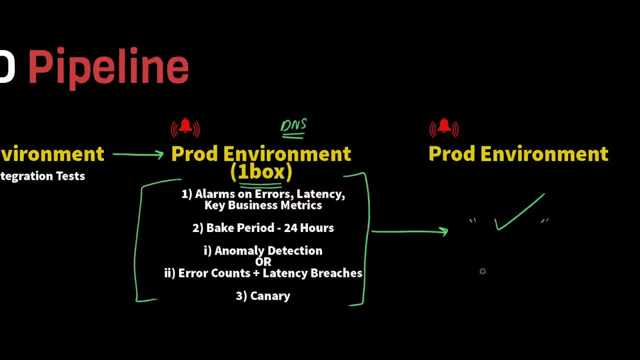 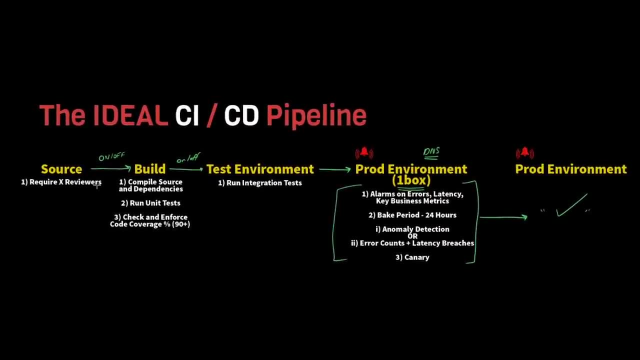 everything is working correctly. So that is kind of what I think a ideal CI CD pipeline looks like. So just to recap, we have the source requiring the reviewers, We have the build steps, We have the test environment, We have an optional kind of pre-prod step in between here, If you want. 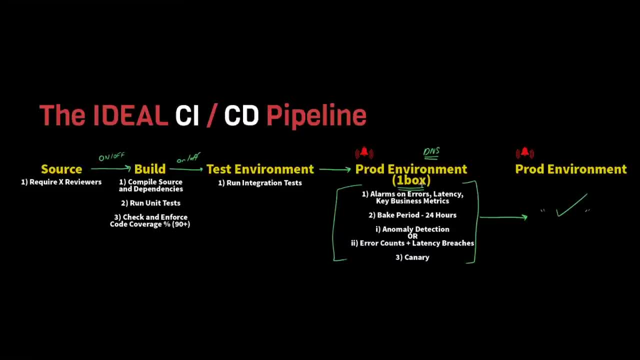 to add some additional redundancy. we have that production, one box which serves a portion of the traffic, And we have a full-blown prod environment which serves the remaining remainder of the traffic. So one thing I also wanted to talk about really quick is just the 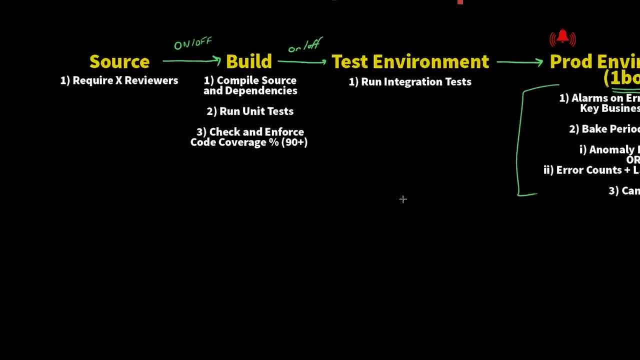 developer experience. Like how should the developer experience fit into all of this? Maybe I'll just draw it down here just to kind of explain a little bit. So the way that these stacks should be set up, like in your service, say, it's order service that manages the creation. 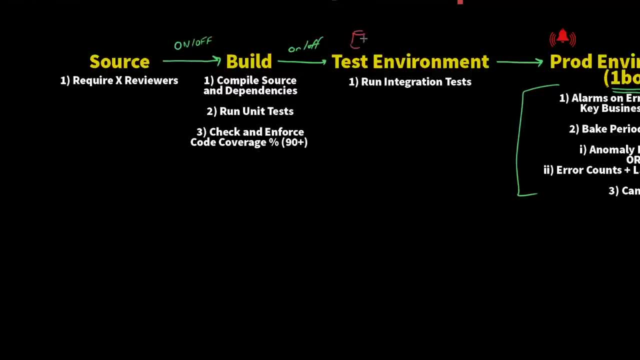 of orders like: the test environment has its own database, right, That's the test database And your prod environment has its own database over here, right? So these things are completely separate from one another. the test and the prod environment. They have completely different. 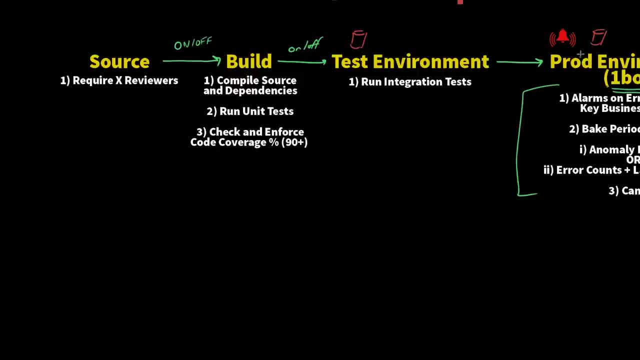 resources that are created in the cloud or created in your data center, Now in the dev environment. so, in the dev environment, ideally, how it should work is that you should have, like you as an individual here, should be able to have your own version of the database that's associated. 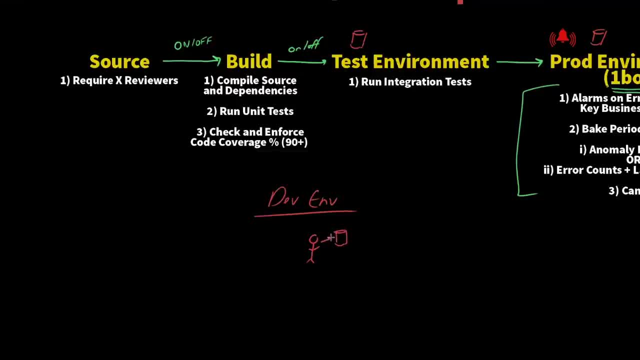 with the test environment And this is going to be like completely local to you. So when you spin up your application, say the test environment, you should be able to have your own version of the database that's associated with the test environment. So in the dev environment, say this: 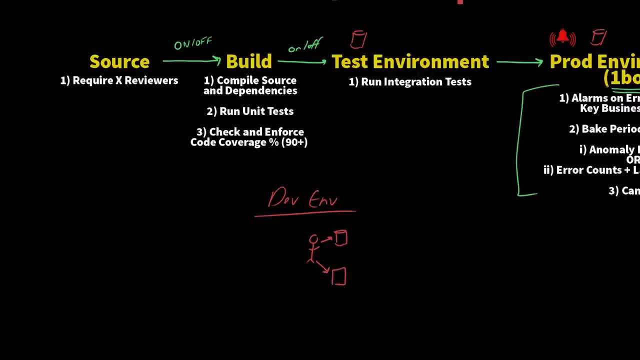 thing is order service over here and you spun this thing up. your order service local version should know to connect to this, also local version of the database And, in addition, like this, this database would be in the cloud somewhere, assuming you're using something like AWS or GCP. 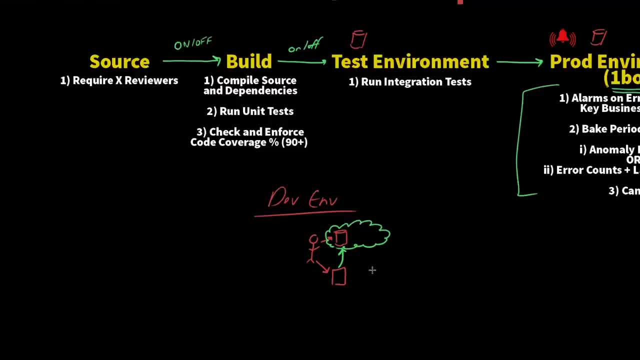 or Azure or whatever any other infrastructure that's required for your system to behave. maybe it's an SNS topic, maybe it's a Lambda function, maybe it's- I don't know. whatever you may have that should also be in here, So like you can have your own version of the database. 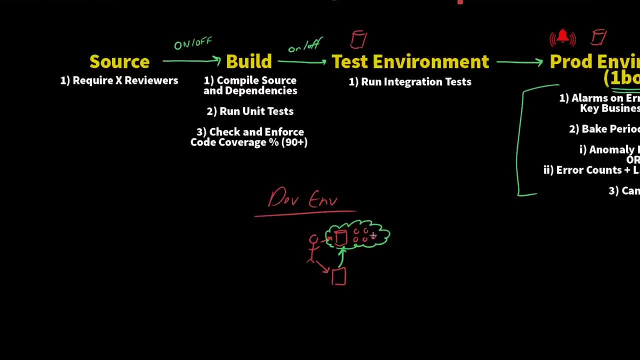 you can have multiple different pieces of infrastructure. that are all in here, But they're all specific to you, specific to each developer, And then in tandem, in your test environment, you also have all this infrastructure right, And this stuff all exists in the test. 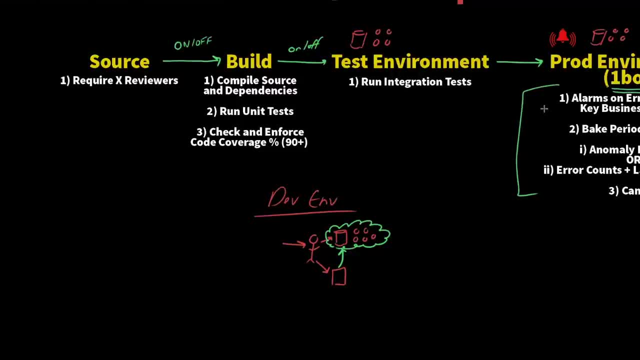 environment, And similarly it also exists in the prod environment. So that's the idea here: the dev environment should be completely isolated, ideally in a separate AWS account, so that you kind of reduce the blast radius in case anything goes wrong. One thing I just 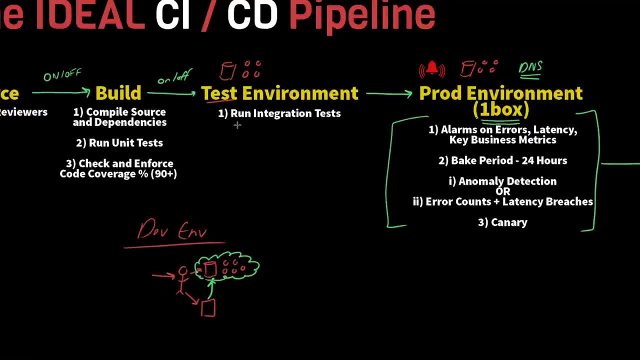 remembered I forgot to mention this- should be a separate AWS account. So if you're using a test environment, it should be in its own AWS account. prod environment should be in its own AWS account. prod in one box can share the same AWS account. I don't think that's a big deal. 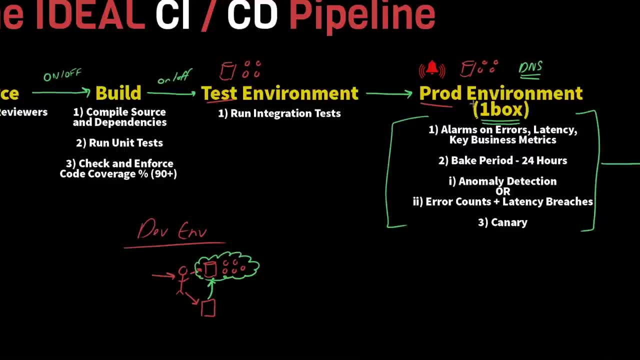 But ideally, each environment and region combination should be in their own. And that also reminds me of something else: What if now you have regional deployments, Like: what if you have a stack that's for North America, one that's for Australia and one that's for I don't know? 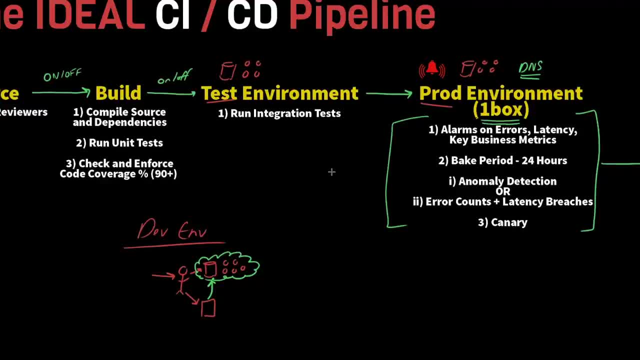 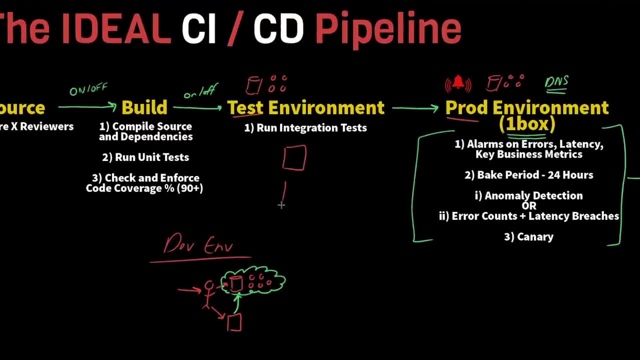 let's say Europe. So how should this thing change? Well, it doesn't really change that much, except that you have, like, in your test environment, you have three different environments that are within it and they're all regionalized. So you have your NA one here. 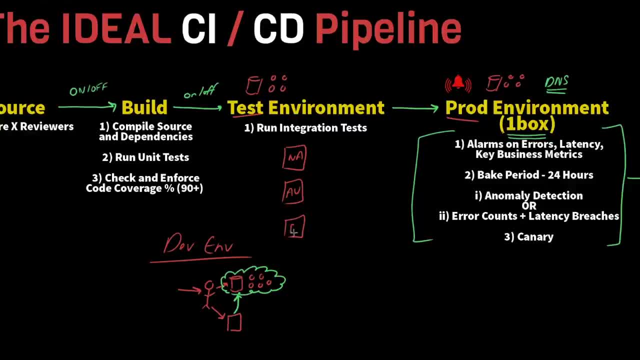 you have your Australia one here, AU, and then maybe your EU one here, And when you build- let me get that green again- when it goes to your test environment, it's going to go to NA and then from NA it can go to AU and then from AU can go to EU. Or, optionally, you can go like: 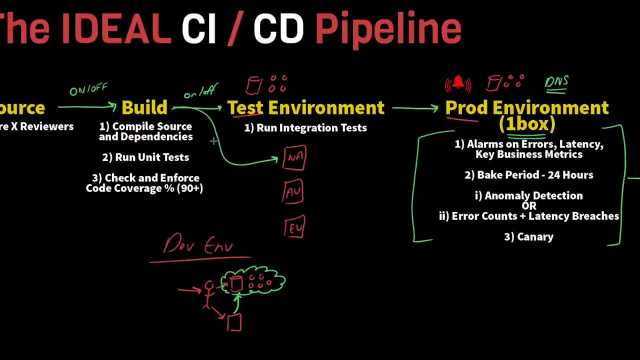 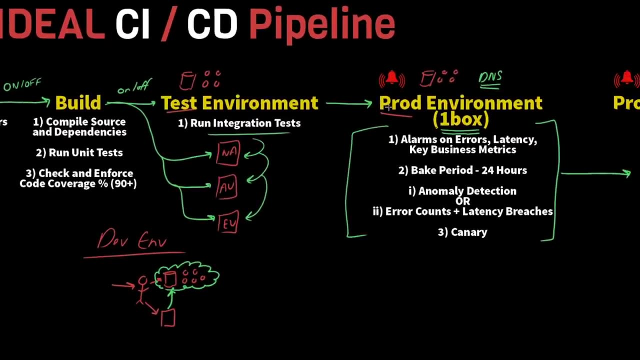 this, instead of having like NA to the next two below it, you can just build and it'll go like in parallel to all of these three at once And then you just run your integration tests against each of these things here, So against your NA, EU and AU, And similarly here, like in your prod. 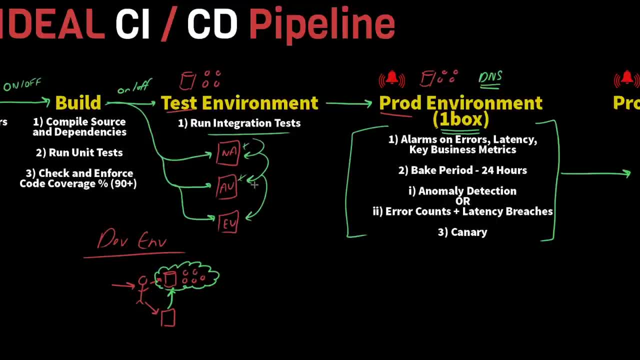 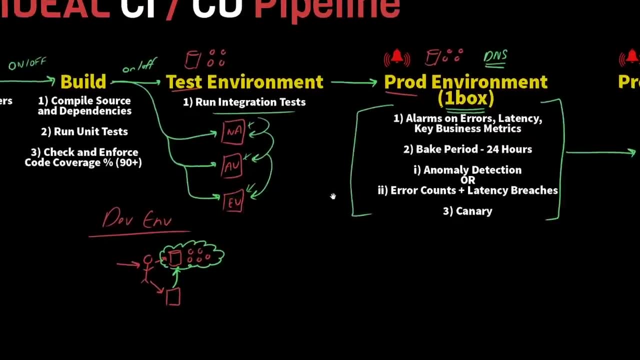 you'd have the one box for NA, for AU and for EU. You have your one box for all of them and for your final production environment as well. So this is the idea of what I would consider to be kind of a gold standard, And of course, you can always add, like more. 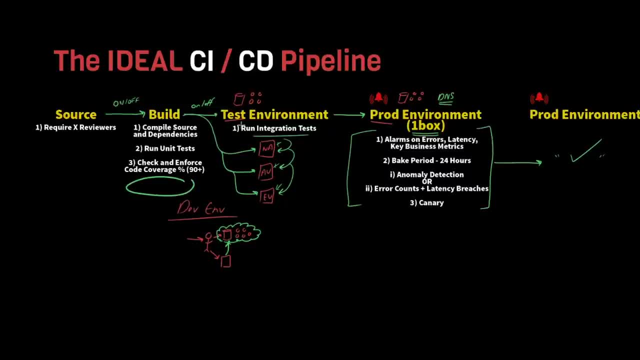 things here in the build steps. You can add more things here in the test environment if you want to do like functional tests or anything like that, But this is a really good starter template. Now currently at my workplace I have like internal tooling that I take for 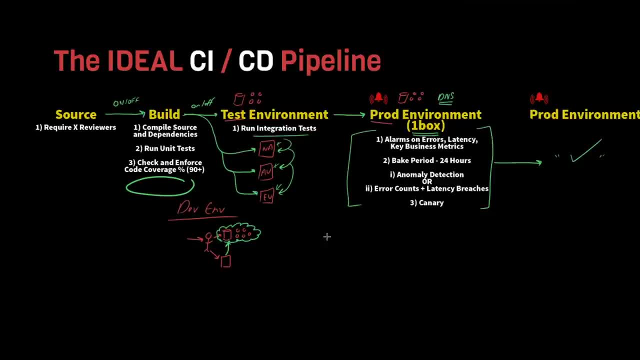 granted that provides like similar functionality to this. So what I'm trying to do in my off time is basically build this entire setup on AWS, And I have a video that I'll put on the right hand side here and in the description section. 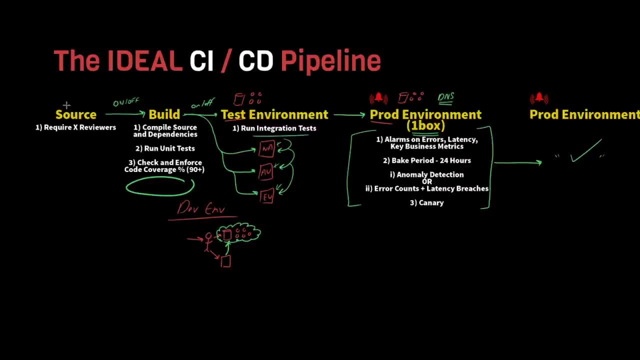 where I'm getting started with this process. So I've currently set up, like the source stage and the build and the deployment to the test and the prod environment, But I haven't done, like all of you know, this stuff where it runs. the unit test does all the code coverage. 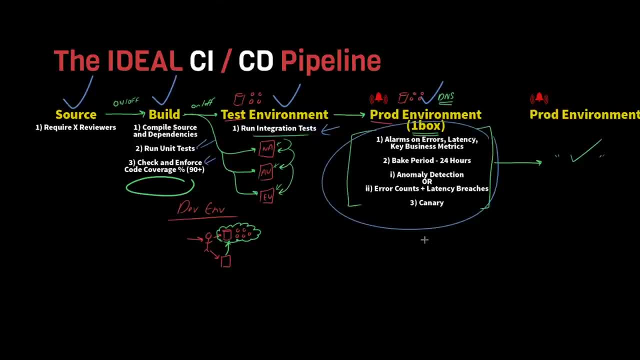 does the integration tests? I haven't done any of this, So this is what I'm currently trying to figure out, So you can follow along with me as I learn and apply that And I'm going to be trying to do basically everything that I'm doing right now and I'm going to be trying to do basically. 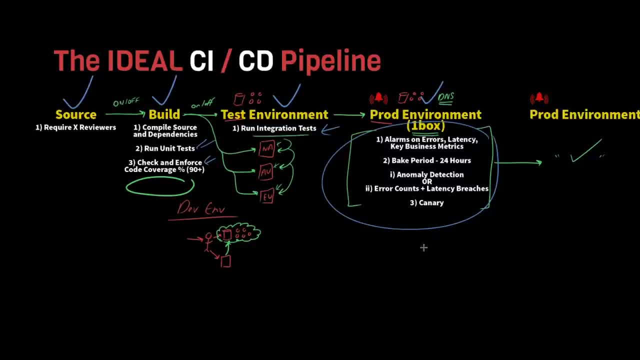 everything that I'm doing right now. So I'm going to be trying to do basically everything I'm doing that I did in this video on AWS using CodePipeline, CodeCommit, CodeBuild, CodeDeploy- all the code things- to see if I can get it to a point where I'm happy with it. But this is what.